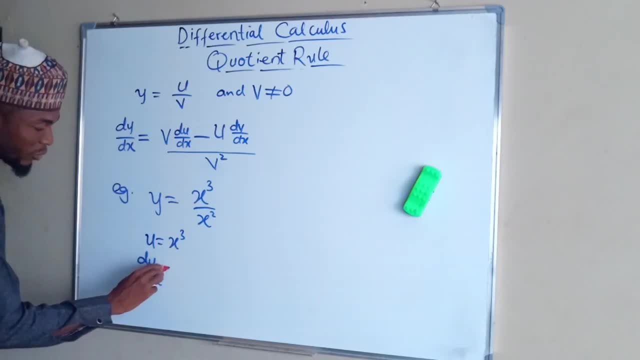 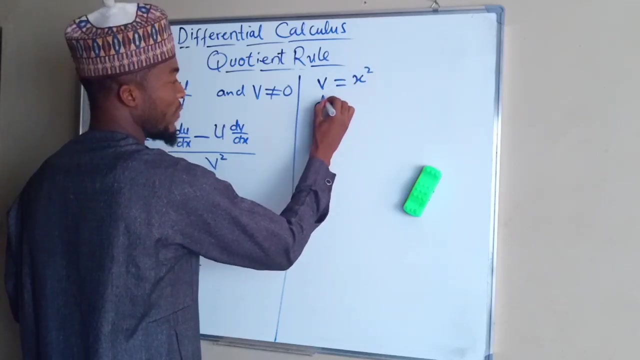 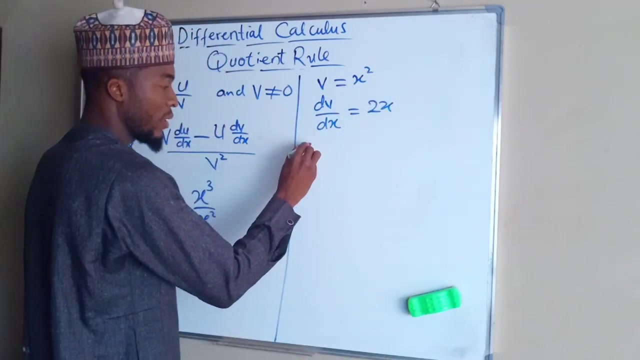 then du over dx will be equal to 3x squared. Then for v equals x squared. therefore, dv over dx will now be equal to 2x. dy over dx will be equal to. you are going to substitute. 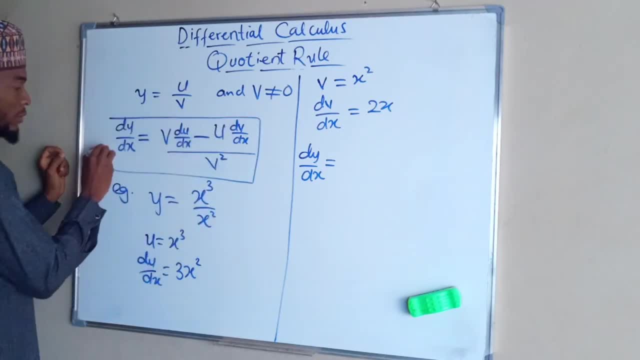 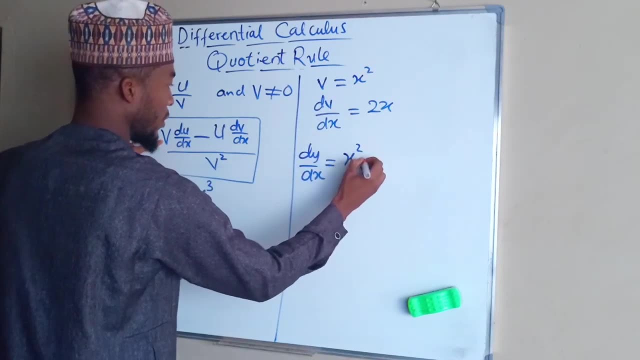 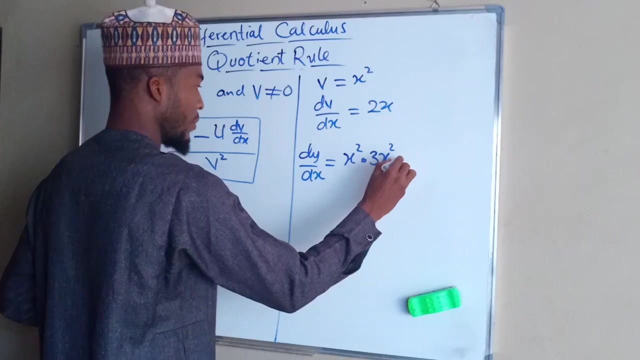 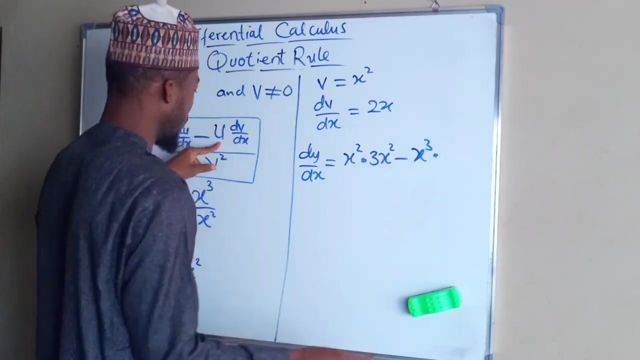 from this formula dy over dx is this: our v is x squared times du over dx, which is 3x squared minus. u is x cubed x power 3, times dv over dx, which is 2x. 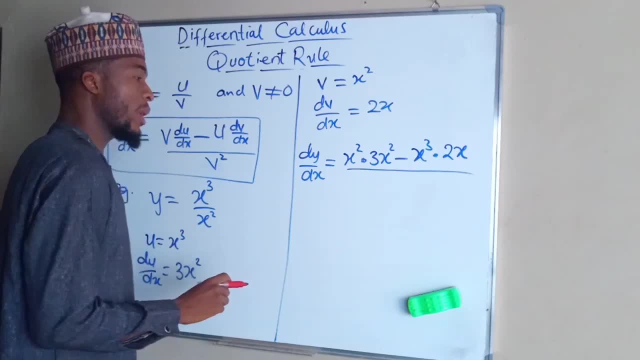 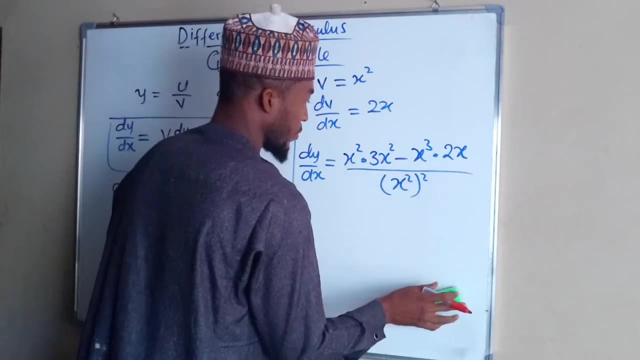 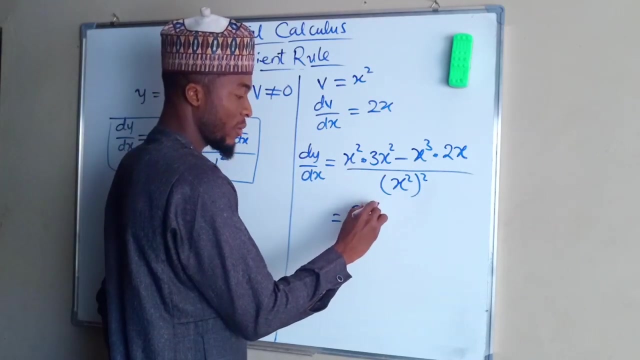 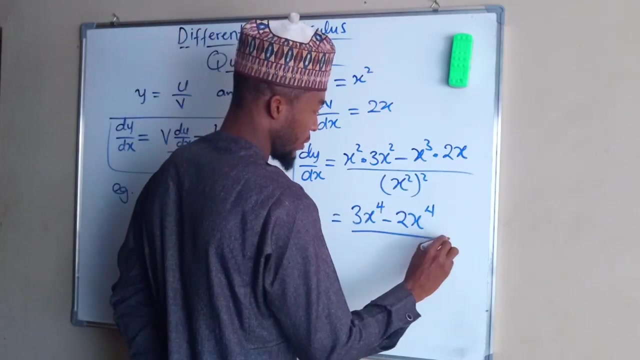 Di윈 over dv. I run this prime over box expression divide by v squared, and v squared is our x squared power 2.. Now we simplify: This is 3x power 4, minus this one, this is 2x power 4.. 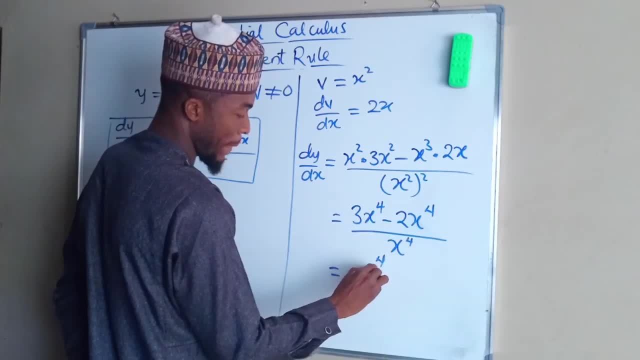 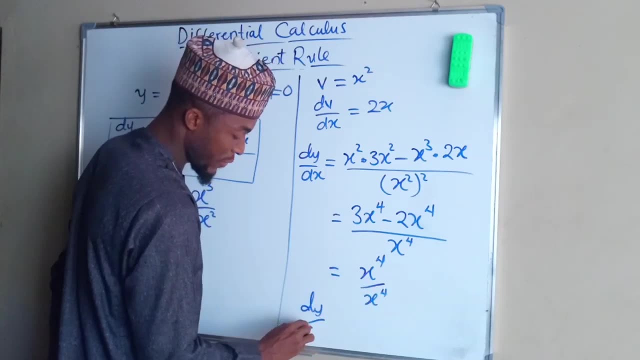 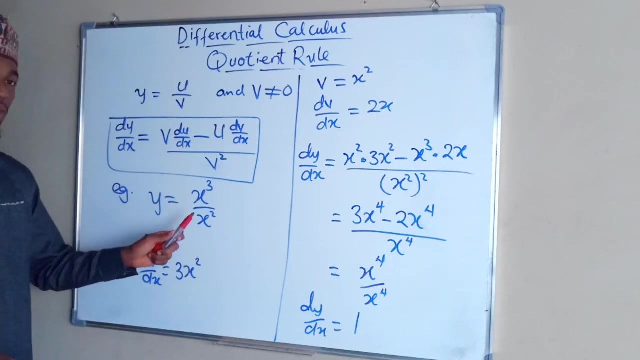 that equal to this minus this, which is just x power 4 divided by x power 4. and finally, dy over dx will be equal to 1, because the numerator and denominator are the same. another way you can differentiate this is to simplify. by simplification this is what i mean from laws of indices: x power. 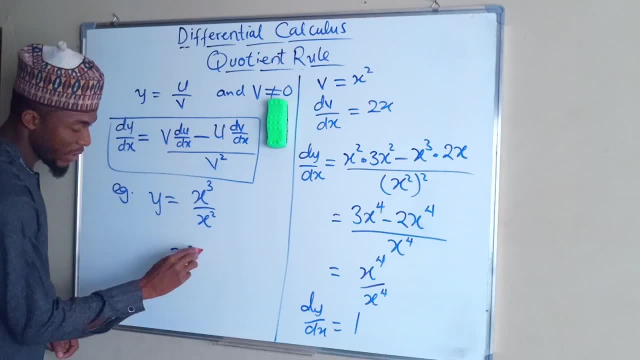 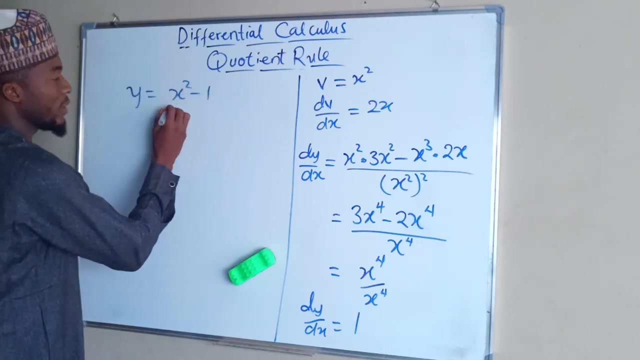 3 divided by x, power 2 will be x, and you know that dy over dx is going to be 1. and which is this? suppose y equals x squared minus 1 divided by x plus 1. no matter how smaller or higher the degree of the exponent is, the methodology for solving the differential equation remains the same. 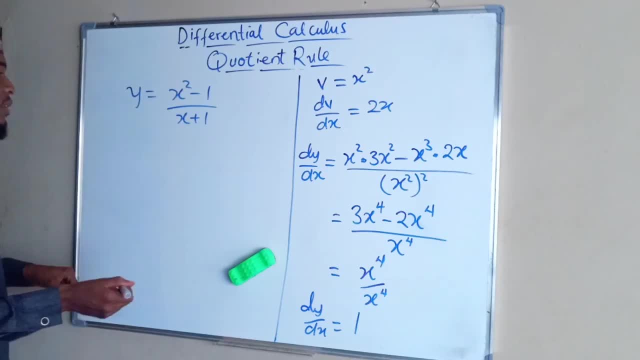 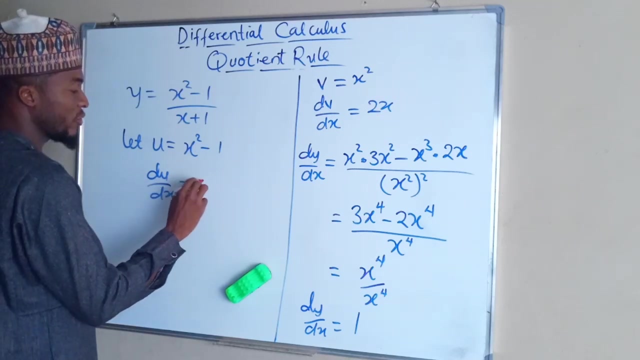 so i'm not going to be using higher degree of exponent. there are two ways in which you can solve this. you can first of all simplify, or you can just apply your quotient rule. for quotient rule, you let u equals x squared minus 1. you differentiate u with respect to x and this will give us only 2x, the v equals. 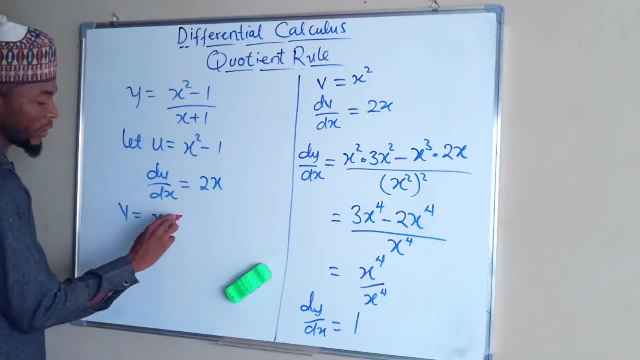 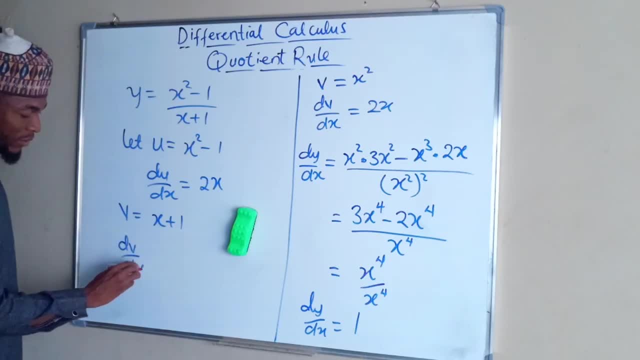 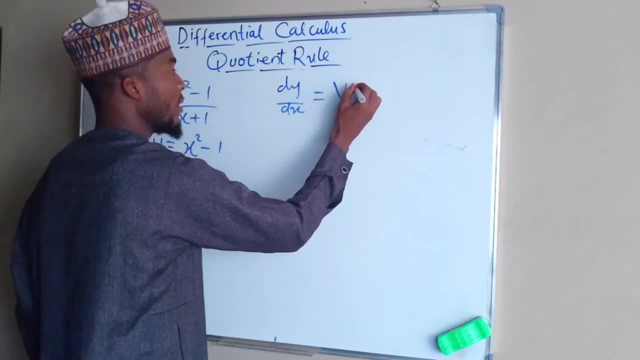 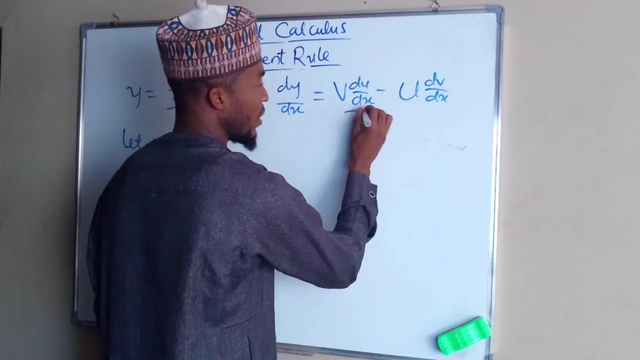 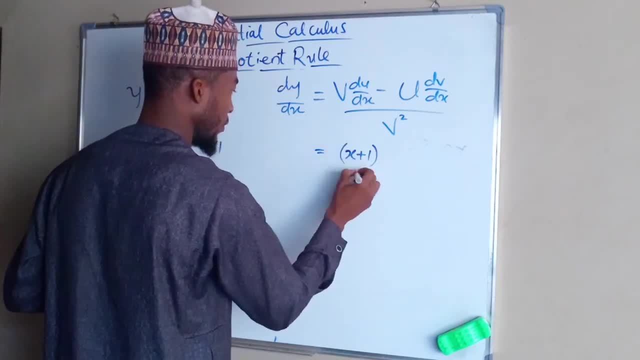 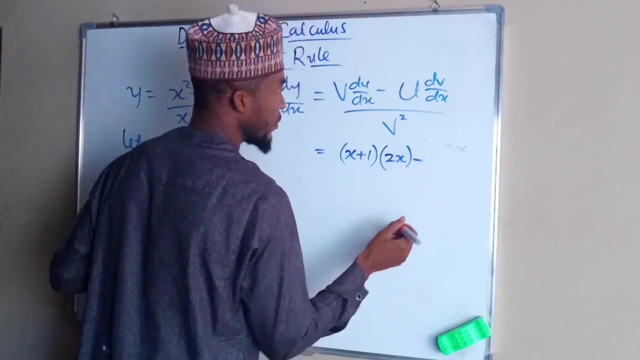 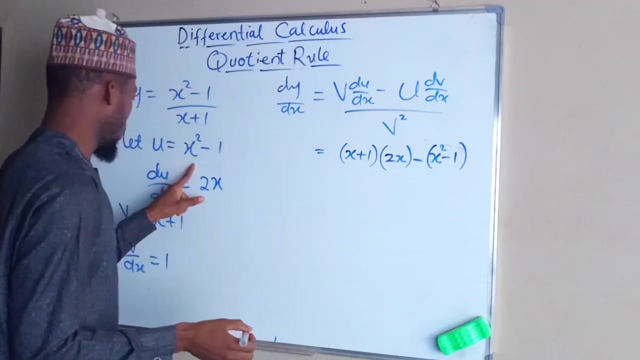 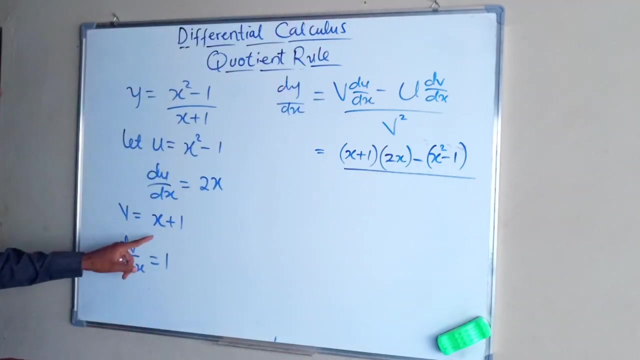 v is x plus 1, du over dx, du over dx is 2x minus u, is x squared minus 1, x squared minus 1, then dv over dx is 1, so 1 will not change the value divided by v squared, which is x plus 1. 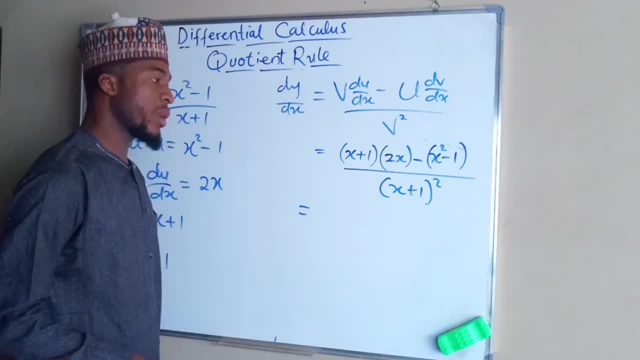 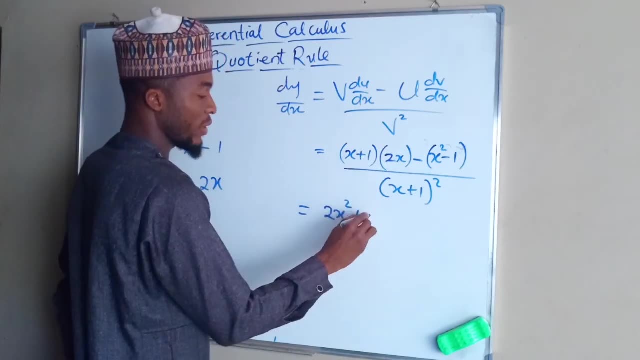 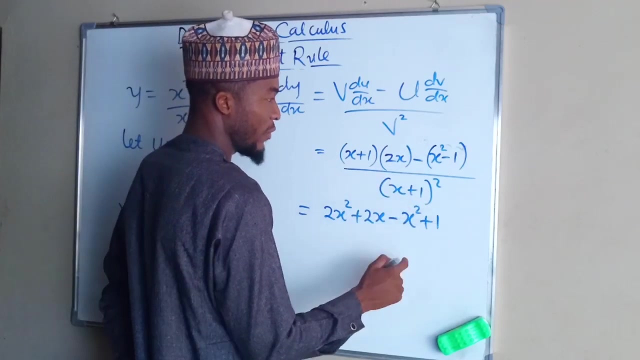 squared. let us expand the brackets. 2x 2x times x is 2x power. 2 plus 2x times 1 is 2x minus x, squared plus 1. if you expand the bracket, that is what you are going to have. 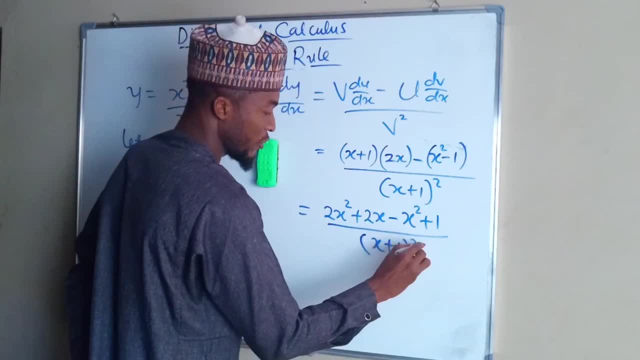 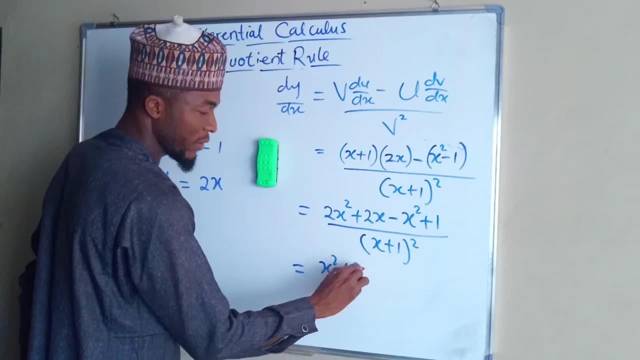 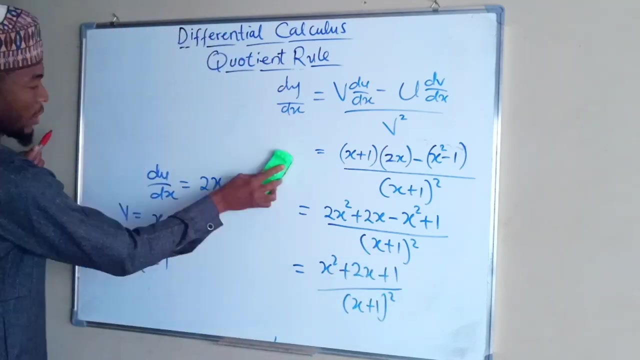 divided by x plus 1 squared, then 2x squared minus x squared is x squared plus 2x plus 1 divided by x plus 1 squared. from here you know that this is a quadratic function which is also a perfect square quadratic function which you can factorize as